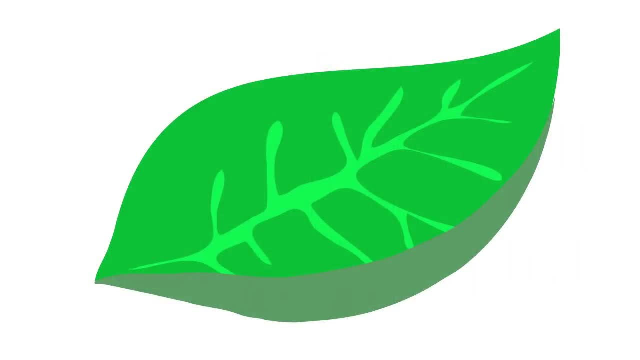 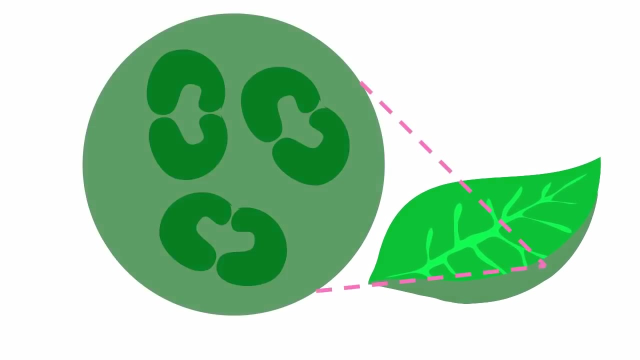 have a large surface area so they can trap as much sunlight. What else do we need for photosynthesis? Carbon dioxide. That's where the bottom of the leaf comes in. It's got these little pores called stomata, which open up so carbon. 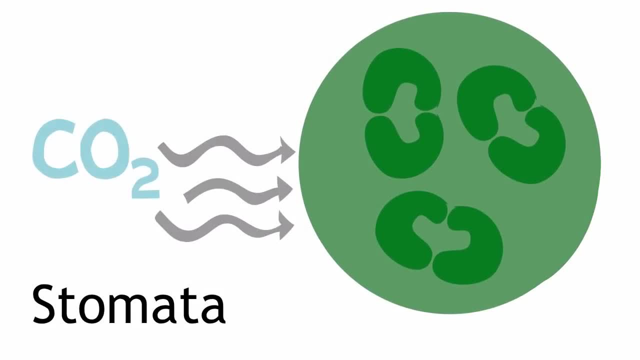 dioxide can diffuse into the leaf. They're controlled by sausage-shaped guard cells which open up to let carbon dioxide in. but they can also close the stomata to prevent other things, like water, from escaping. So the carbon dioxide comes in through the stomata. 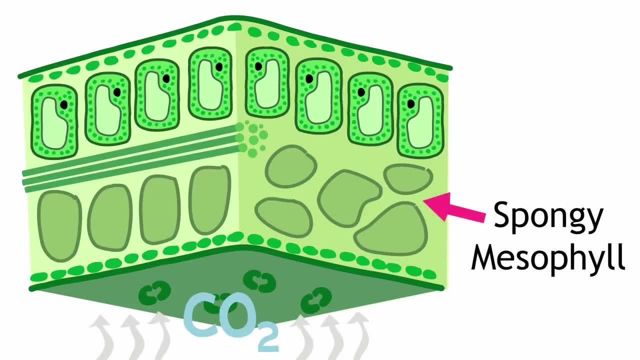 makes its way through the gaps and then airs it into the leaves. So the carbon dioxide goes into the primary layer of cells called the spongy mesophyll at the bottom part of the leaf and then heads up to the palisade layer for photosynthesis. Leaves are thin. 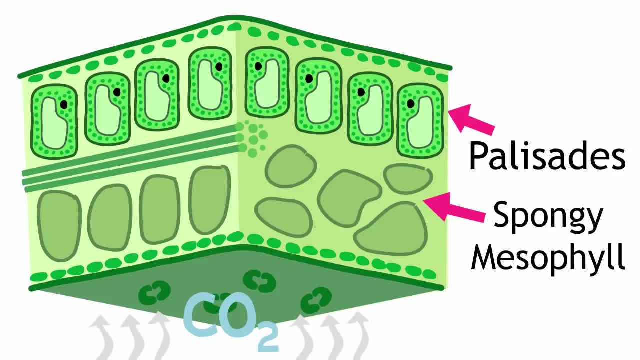 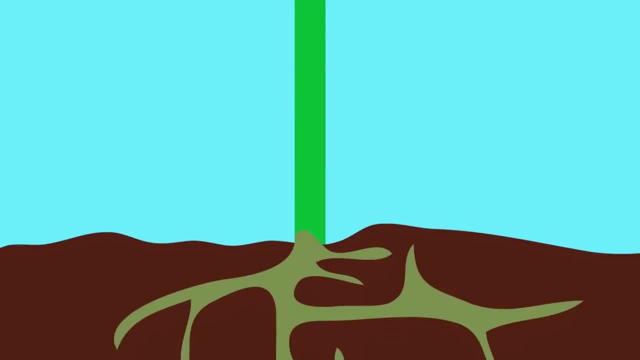 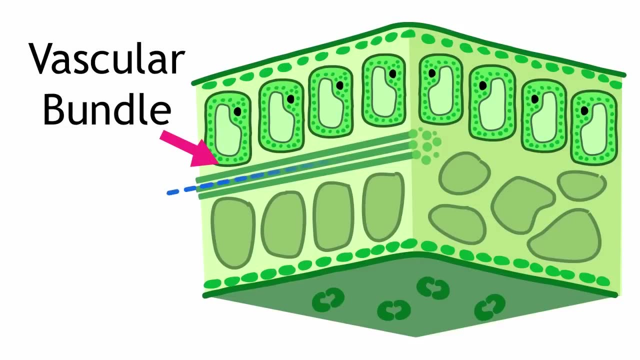 so that the carbon dioxide won't have too far to travel. So we've got sunlight and carbon dioxide. now What's left? Water. Water comes up through the roots and stem and enters the leaf through a vascular bundle which contains a hollow tube for water transport called the. 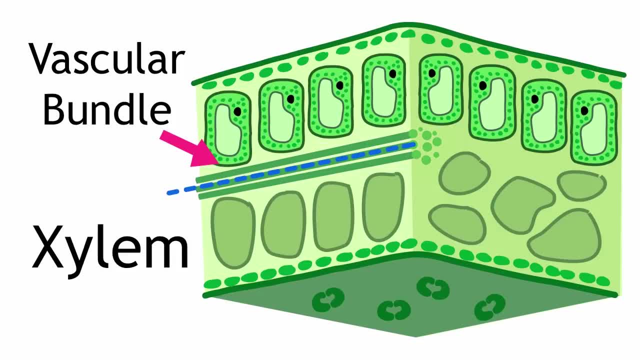 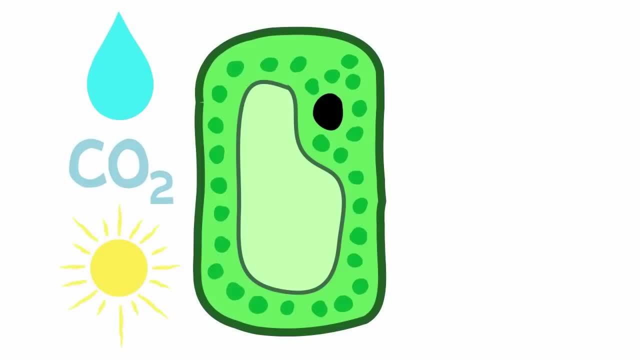 xylem. Look at how the vascular bundle spreads out in the leaf to form veins so that it can spread water throughout. So now the leaf's palisade cells have water, carbon dioxide and sunlight- All they need to photosynthesize and make glucose, their food and oxygen. But how does 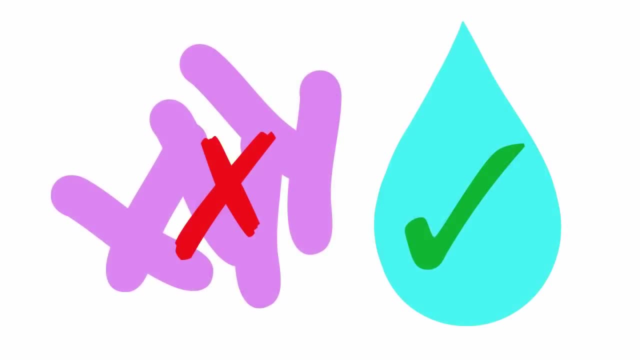 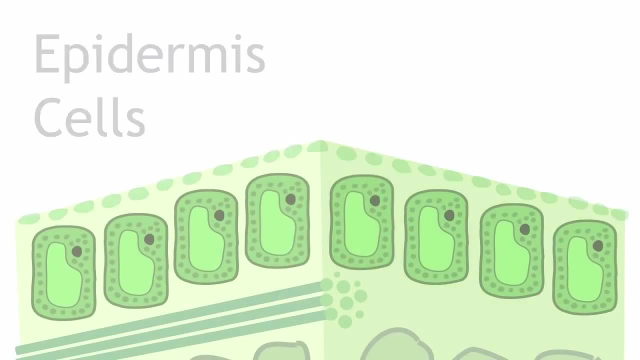 the leaf prevent unwanted intruders like bacteria from getting in and stop important reactants from escaping. Above the palisade, mesophyll and below the spongy mesophyll are epidermal cells which produce a waxy coating called the cuticle. The cuticle seals up the leaf. 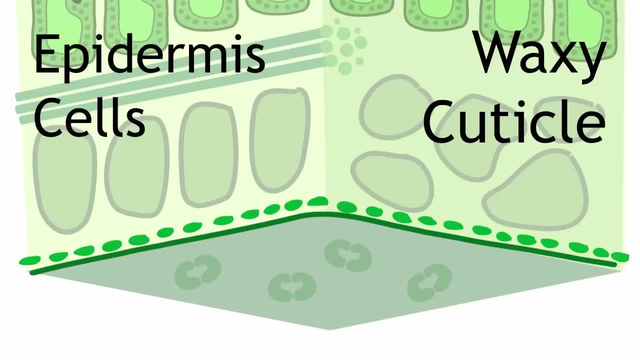 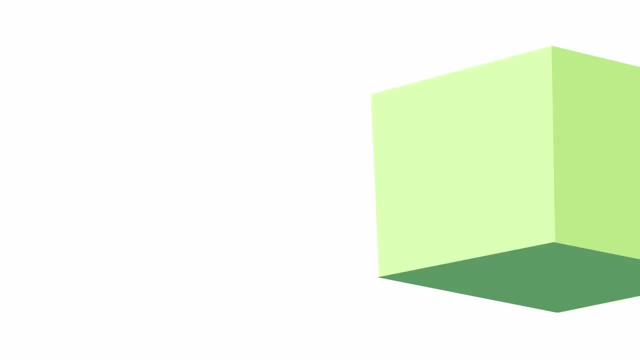 so that the only way in and out is through the stomata, which are regulated by those guard cells. Now let's go back through the parts of a leaf. from top to bottom We've got the thin waxy cuticle, then the epidermis cells. These basically make up the leaf's skin. Then comes the chlorophyll-rich 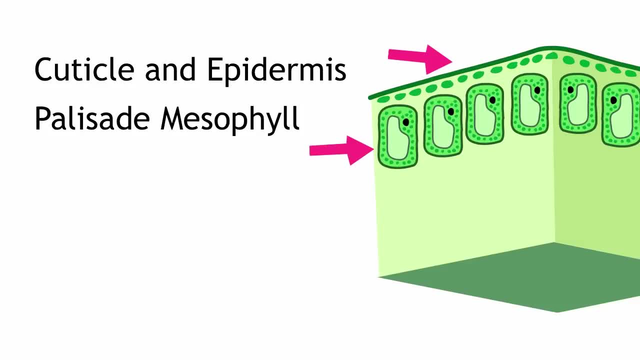 palisade mesophyll where the bulk of photosynthesis occurs. Below that's the spongy mesophyll which have plenty of space in between them for reactants to move through Through. that space stretches the vascular bundle with xylem to transport.